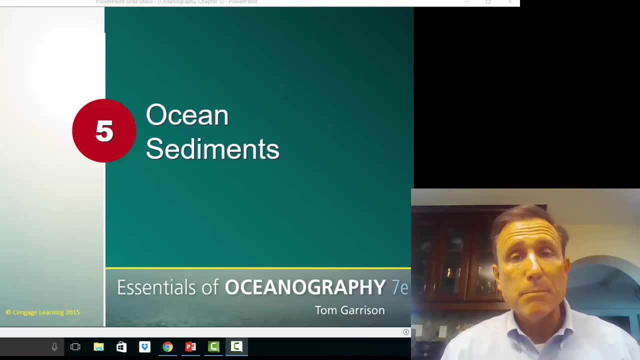 ocean sediments that we've begun to understand. concepts like plate tectonics and ocean basin construction, the ability for the earth to generate new crust and to consume old crust, And also ocean sediments have been very valuable in helping us to understand past climates. So 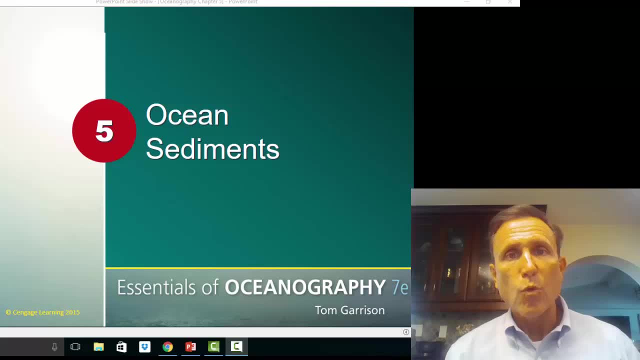 paleoclimatology, knowing when it's been colder and when it's been warmer on the earth's surface, knowing when ice sheets cover the earth and knowing when sea levels have been higher and lower. So ocean sediments- very important stuff. First, we'll start out with an overview of what 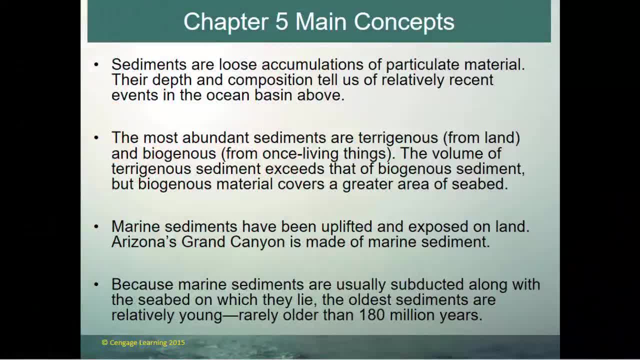 we're going to learn in Chapter 5.. All right, Chapter 5, main concepts. First, sediment. What is sediment? Loose accumulations of particulate matter. The depth and the composition of sediment tells us of relatively recent events in the ocean basin above, But very, very deep. 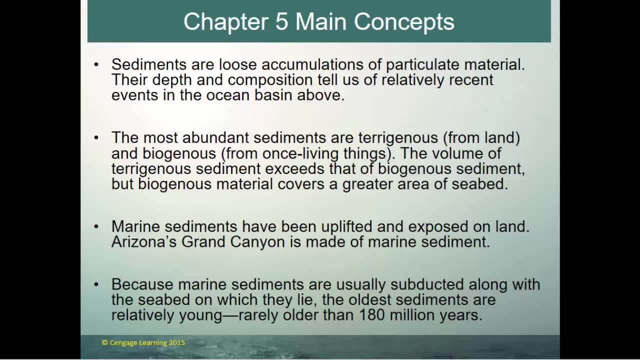 layers of sediment buried under lots and lots of other material can tell us about what's happened in the distant past. Number two: the most abundant sediments are pterogeneous, That's from land, And then biogeneous, which are from once-living creatures, Once-living organisms in the ocean. 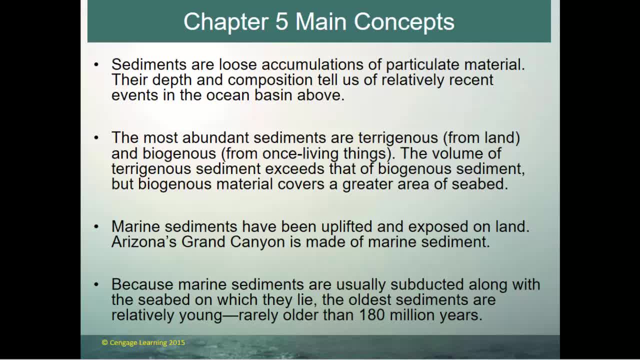 sediment. The volume of pterogeneous sediment exceeds that of biogeneous sediment, But biogeneous material covers a greater area of the seabed. The sediment from land basically covers the continental shelves and the continental rise. The biogeneous sediment is what covers the abyssal. 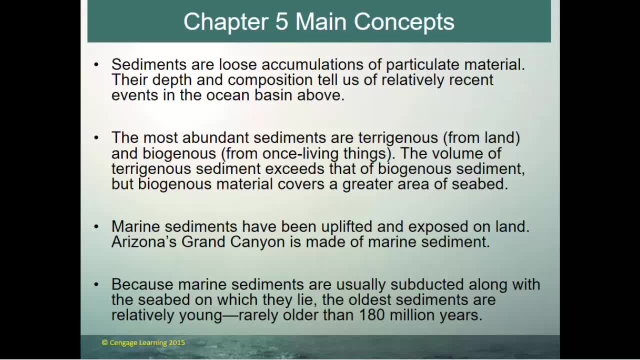 plains. Number three: marine sediments have been uplifted and exposed on land. So sediment doesn't just stay on the ocean floor, It's covered by more sediment. Eventually it's compacted and lithified, turned into sediment. So sediment doesn't just stay on the ocean floor, It's 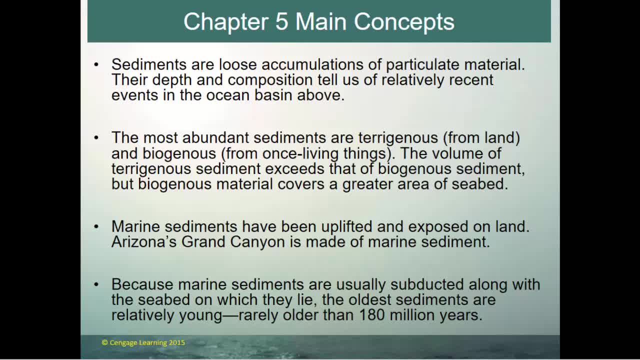 turned into sedimentary rock And eventually, due to plate tectonics, that sedimentary rock can be uplifted and exposed on land, much like what we see in Arizona's Grand Canyon. Number four, because marine sediments are usually subducted along with the seabed in which they lie. 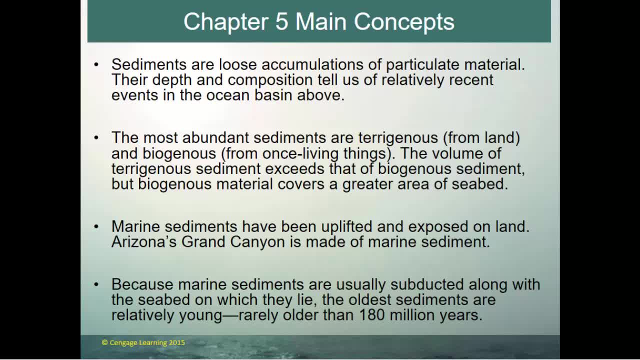 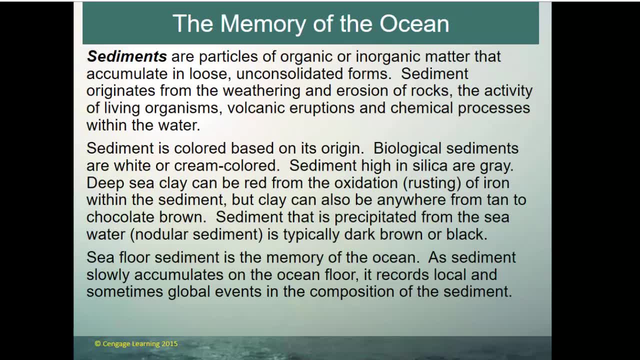 the oldest sediments are relatively young and rarely any older than about 180 to 200 million years of age. So sediments are oftentimes referred to as the memory of the ocean, Because sediments tell us what happened in the ocean basin above in the distant past. 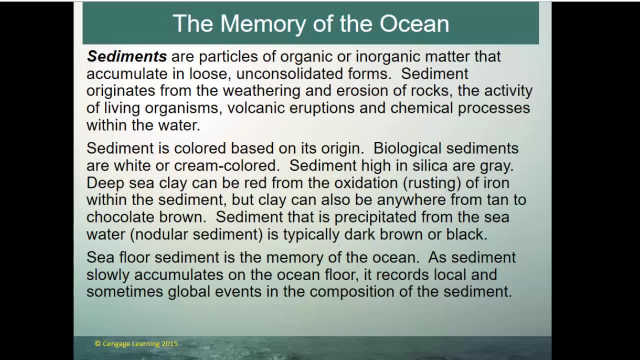 Sediments are particles of organic and inorganic matter – living and nonliving matter – that accumulate in loose, unconsolidated forms. Unconsolidated means it's not compacted and lithified into rock, So sediment is not rock. It is a different thing. Sediments can become. 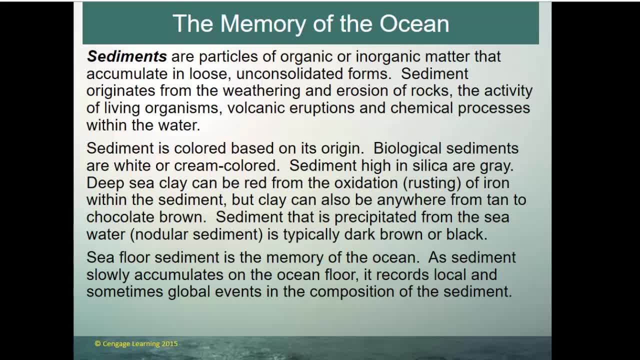 sedimentary rock when it is compacted and lithified- Lithified essentially just means cigarettes to bottles loaded into the ocean floor with ash and ash and put into surfacerajcotes昆 of unconsolidated materials together. So sediment originates from the weathering and erosion of 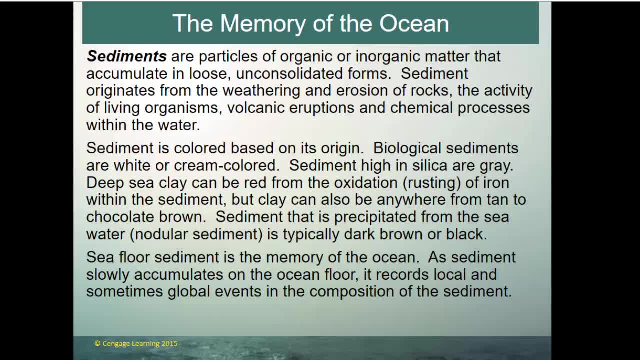 rocks and the activity of living organisms, also from volcanic eruptions, and the chemical processes within water. All of these processes can generate sediment. Sediment is essentially color based on its origin. The color of the sediment is typically an indication of its origin: Biological sediments. 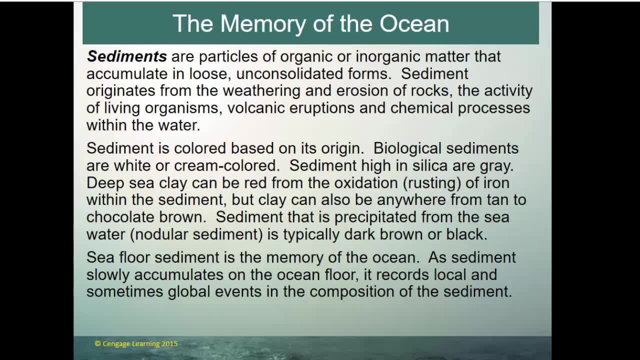 are white or cream colored and that reflects the shells of biological creatures. Sediments that are high in silica tend to be gray. Deep sea clays can be red due to the oxidation or the rusting of iron within the sediment, but clay can also be anywhere from a tan to a very deep chocolate brown Sediment. 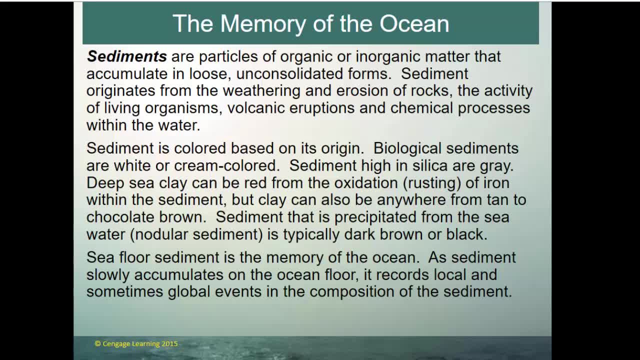 that is precipitated from the sea can be red. Sediments that are high in silica tend to be gray Water itself. nodular sediment is typically a very dark brown or a black. We said that seafloor sediment is the memory of the ocean. As sediment slowly accumulates on the ocean floor, it records. 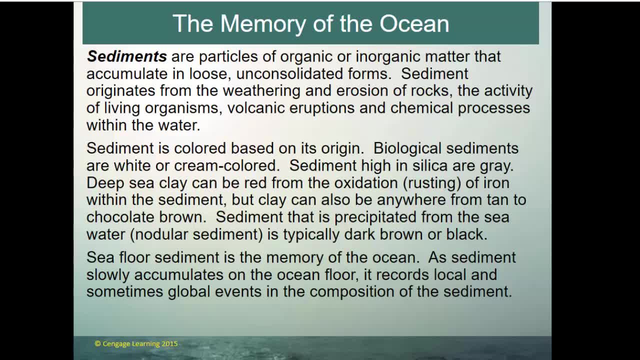 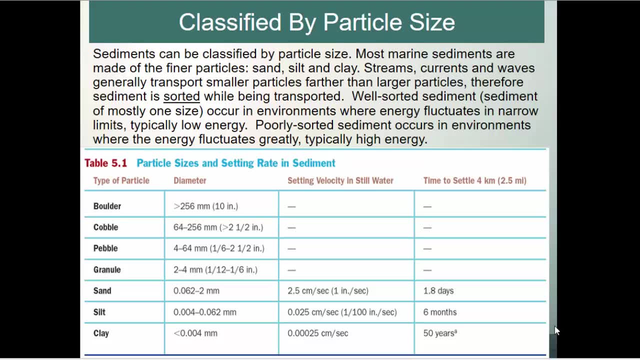 local and sometimes global events in the composition of the sediment. Sediment can be classified by the particle size. Sediments can be classified by the size of the individual particles, with most marine sediments being made of fiber. Sediments can be classified by the size of the individual particles. 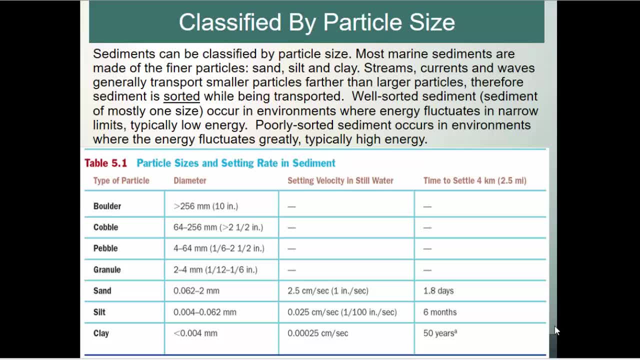 with most marine sediments being made of fiber, streams, and currents and waves generally transport smaller particles farther than larger particles. therefore, sediment is sorted while being transported. well-sorted sedimentpased sediment sediment, mostly one size, occurs in Ankara, la mesura lake, pine, the. 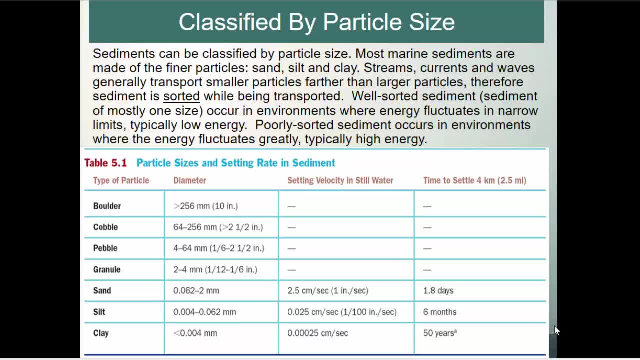 which where? why? in environments where the energy fluctuates greatly, typical in high energy environments. so what does that all mean? well, sediment is transported by medium. that medium is typically going to be water or wind, and the faster the medium is moving, the larger the particles the medium can carry, so a very 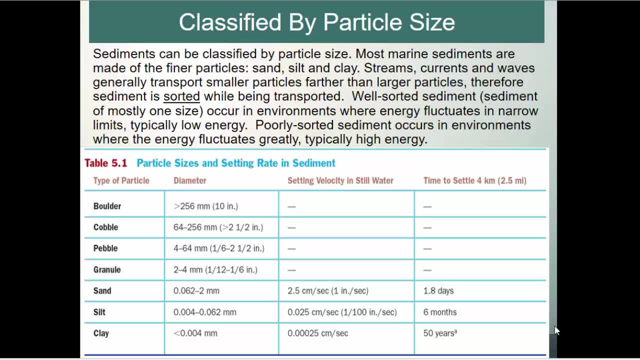 fast-moving stream may carry along with it sediment in the size of clay, silt, sand, maybe even small pebbles, and a rapidly moving stream might even move larger rocks along the stream bed. once that stream empties out into the ocean, it's no longer in a narrow stream channel and the water immediately begins. 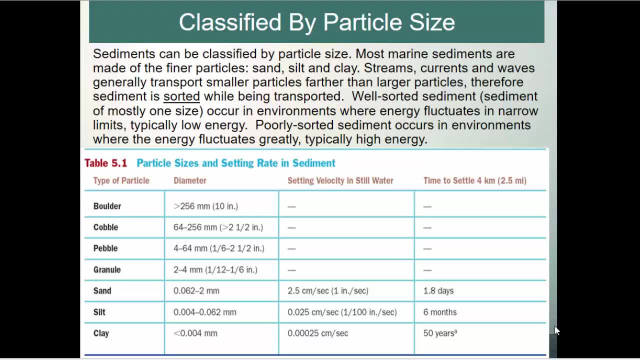 to slow down. as that water slows down, just like if it were with wind, the larger particles will begin to fall out. they can no longer be supported in the medium. gravity takes over and as the water continues to move out- in this case out to sea- and slows and slows and slows again, smaller and smaller particles are. 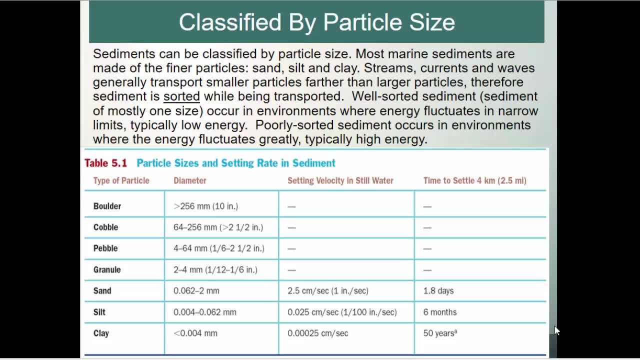 dropping into the ocean, and that's when the stream changes into a water stream out of it, until all that is left is the finest particles, and those are the ones that tend to settle well away from the continental margins, out on the abyssal plain. so if you have a low energy, 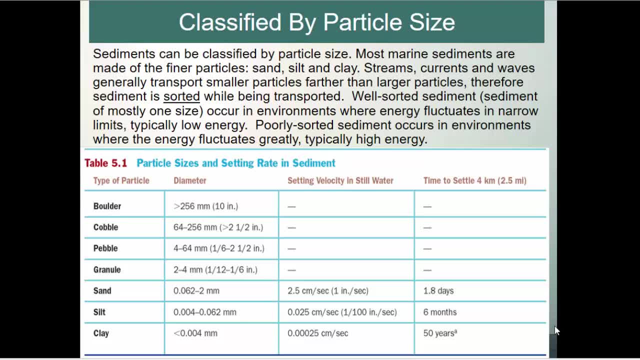 environment, you're basically only going to have sediment of one size, whatever the largest size that level of that energy of the environment can carry. but if you have a high energy environment, like the surf zone, breaking waves and water rushing up and down the coastline or the beaches, 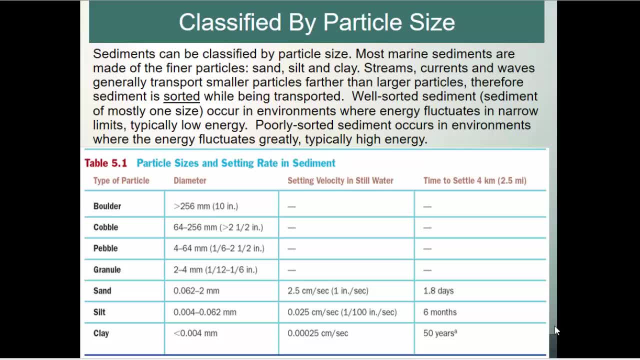 will allow for there to be lots of different or poorly sorted sediments, sediments of lots of different sizes. so that's the difference between your well sorted sediment in the low energy environments and your poorly sorted sediment in your high energy environments. and this table just gives you the particle sizes of sediments and again the sediments we typically find in the 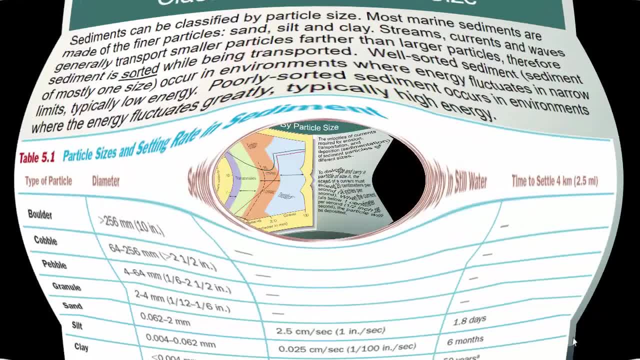 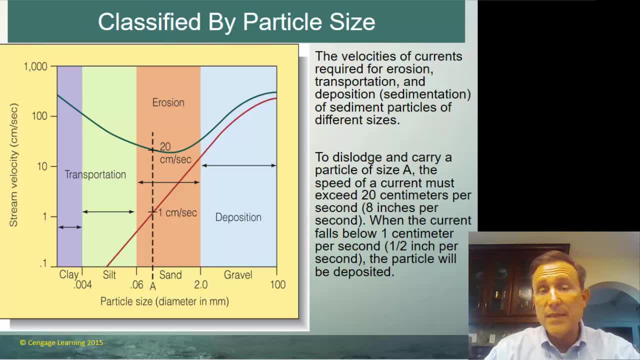 ocean are the smallest: sands, silts and clays. so this chart is going to show us how different sediment sizes are dislodged, carried and then deposited by streams, based on the stream velocity and the size of the particle. so a lot of lines there. it's a little on the confusing side, but if we, if we go, 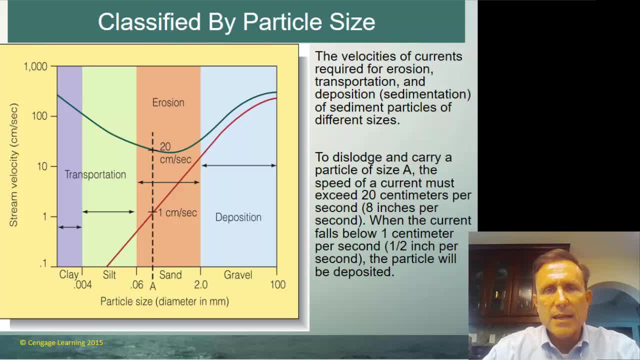 to point a. what this chart is telling us is that a piece of sand the size of point a is going to need a stream velocity of about 20 centimeters per second to dislodge that sand from the stream bed. stream bed velocity falls below about one centimeter per second, then it will no longer hold that size. 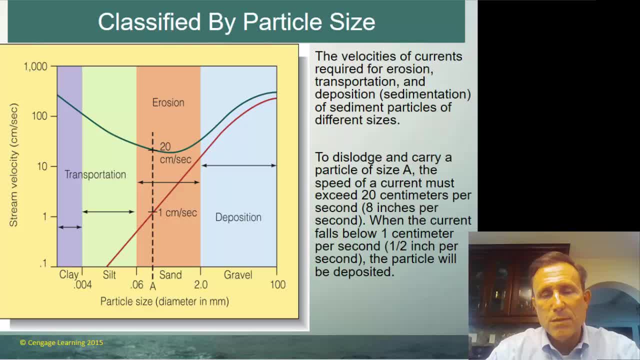 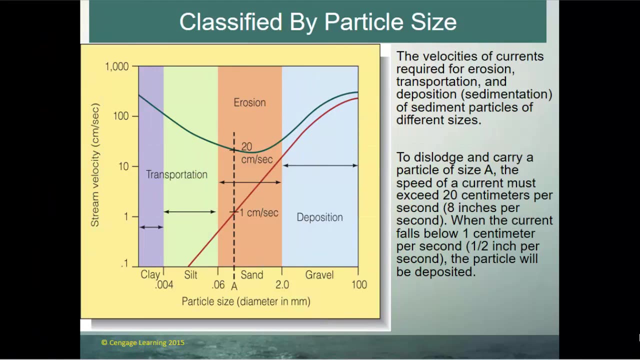 piece of sand and that piece of sand will will drop out and be deposited. so it's interesting if you look at the clays, because the the way clays sit together so well, it takes a very high stream velocity to dislodge them, but it takes a very, very low stream velocity before they'll actually begin. 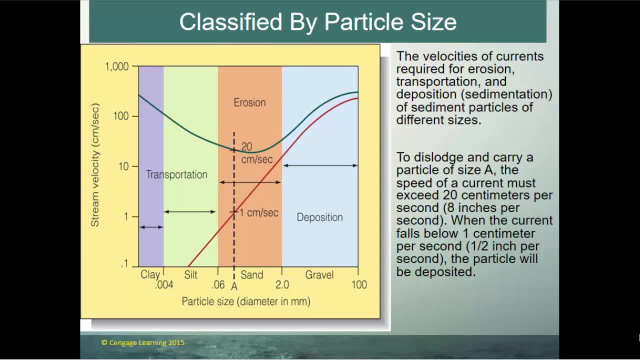 to settle out and be deposited on the sea, in the middle of the sea, so that's going to be a lot of fun. so I hope you enjoyed the video and I will see you next time. on the next video, the surface and, of course, gravel- something very large- is going to take a tremendous stream. 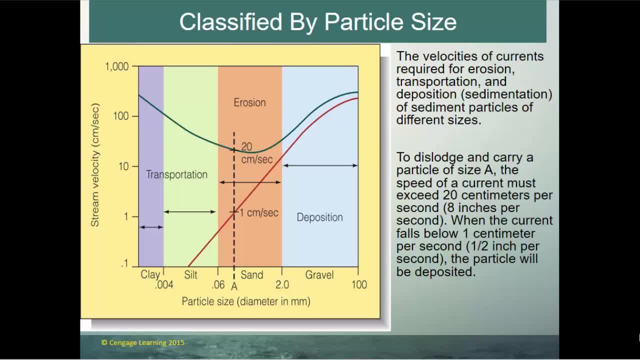 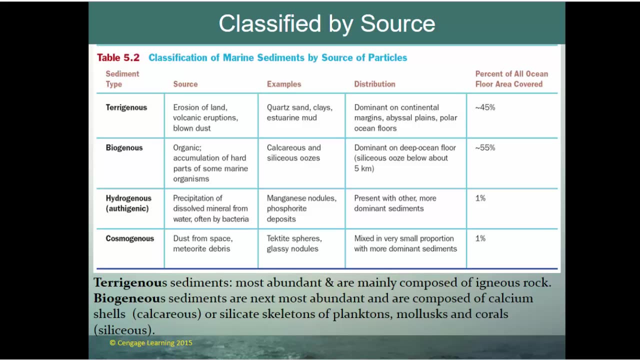 velocity, dislodge it and carry it along. the larger it gets, the more velocity it takes, and very quickly. if that stream velocity begins to to fall, then that gravel will be deposited out of the stream of the stream flow. sediment can be classified by its size. it can be classified by 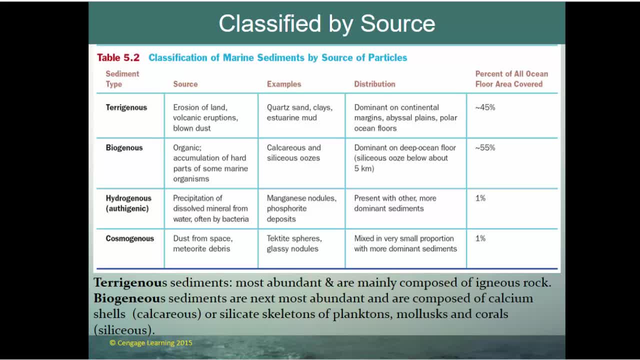 its color, but it can also be classified by its source, and the classification of marine sediments by source is broken down to into teragenous, biogenes, hydrogenous and cosmogenes. and teragenous, with terra being the root of the word, means sediment that comes from land erosion off. 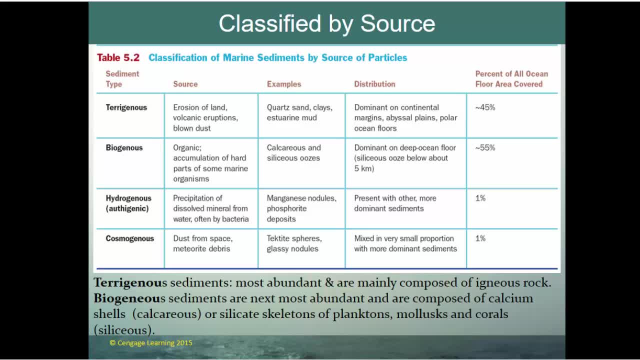 the land, perhaps the debris from volcanic eruptions or blowing dust- and there's actually a tremendous amount of dust that's blown off of north africa out into the atlantic ocean. every year that makes up a large amount of sediment, um, typically quartz sands, clays, maybe echewine mud and, uh, it's dominant on coastal margins, so it's mainly 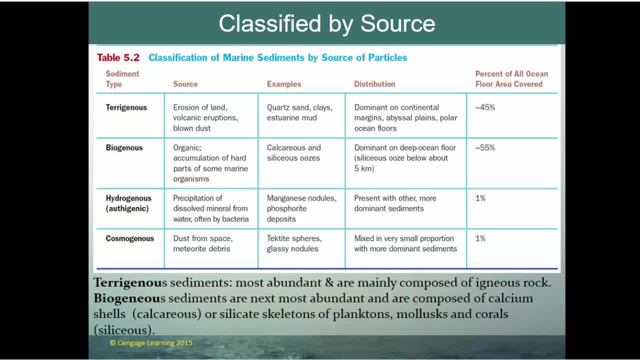 right on those coastal margins, those seaward extensions of the coastline, and then it does get out into the abyssal plains and the polar ocean floors. so the second classification by source is biogenesis, and these are the next most abundant and are composed of calcium shells, um of silicate or silicate skeletons, of planktons, mollusks and chorus corals. so biogenesis is 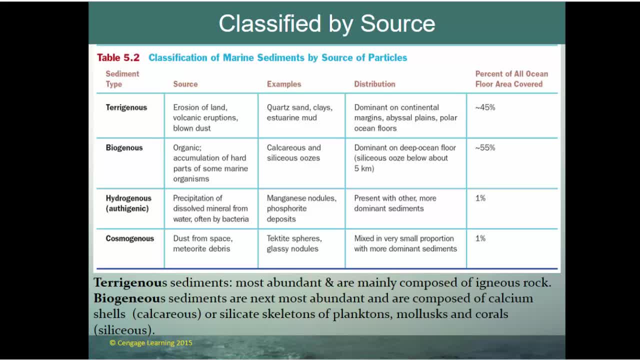 basically the organic accumulation of hard parts of submarine organisms. so pterogenesis is the most abundant, biogenesis is the second most abundant, and you're either going to get these calcium shells or silicate skeletons and they're going to create these, these oozes on the bottom of the ocean floor. that is just a combination of a. 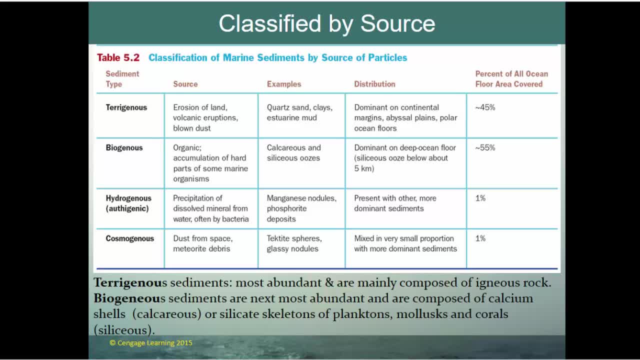 little bit of a pterogenic sediment and then the biogenic sediment. it makes these, the, the dominant on the deep ocean floor and it creates the, the ooze. now, um, you get deeper and deeper underneath the surface and that ooze is lithified, like other sediment, into sedimentary rock. 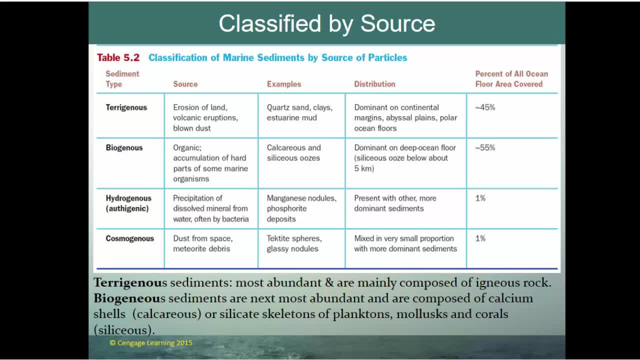 hydrogenous, the precipitation of dissolved minerals from water, typically done by bacteria. it can be manganese, nodules or phosphorite or different types of deposits we find literally on the bottom of the ocean floor where dissolved minerals are precipitated. so they've been dissolved, so they're a solid mineral that's been dissolved into the water. 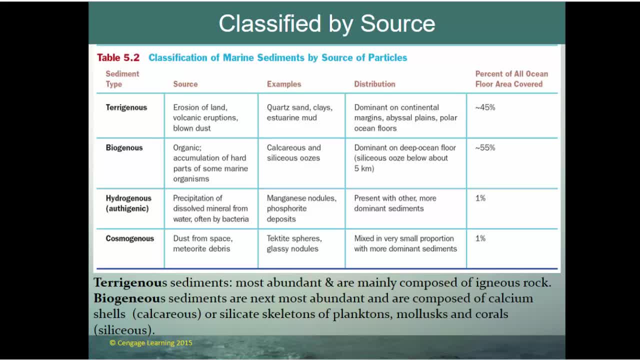 and then, once they're part of the solution in the water, then they can be precipitated out of that solution and become solid again. so cosmogenesis is dust from space and meteorite debris. so, just like dust off of africa, dust from space enters the atmosphere. it falls to earth and starts to 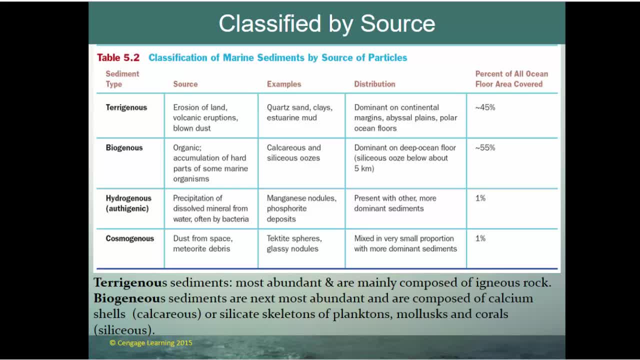 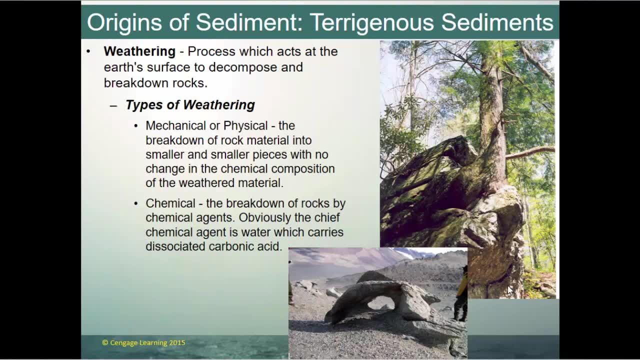 settles into the ocean and you get very small proportions of cosmoginous types of sediments on the ocean floor. Where do we get sediment? If we're talking about terrigenous sediment, we get that from the weathering of continental rock. Weathering is the process which acts at the 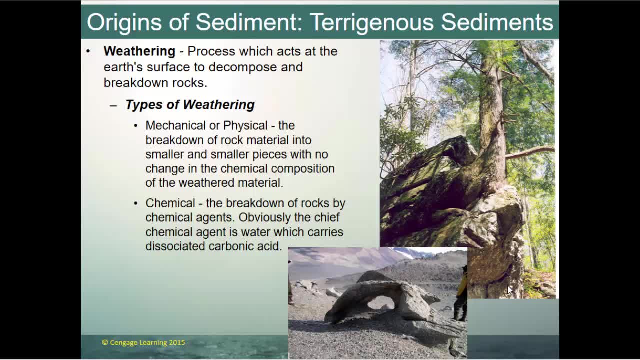 earth's surface to decompose and break down rocks. There's a couple different types of weathering. You have mechanical or physical weathering and chemical weathering. and mechanical or physical weathering is the breakdown of rock material into smaller and smaller pieces, with no change in the 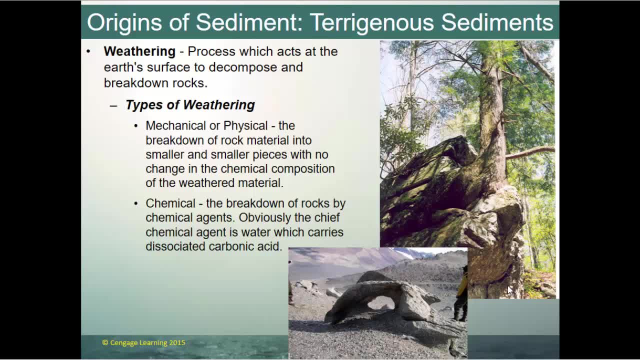 chemical composition of the weather material. That could be from wind, from rain. it could also be from a tree growing into a rock and splitting it into smaller and smaller pieces. Lots of different types of mechanical or physical weathering. Chemical weathering is the breakdown of rocks. 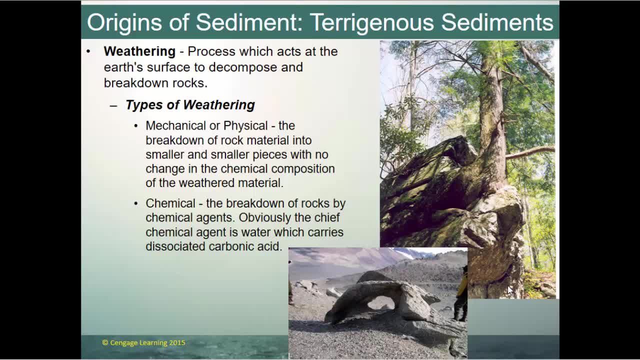 by chemical agents. Obviously, the chief chemical agent is the chemical agent of the rock. The chemical agent of the rock is the chemical agent is water, which carries disassociated carbonic acid, meaning acid rain, A little bit of acidity because of carbon dioxide in the water and that tends to break down rock particularly. 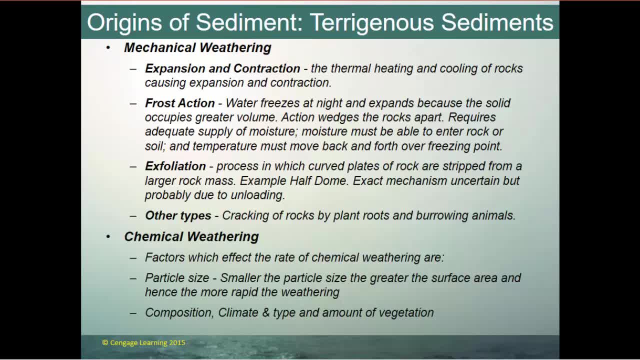 sedimentary rock. it breaks it down quite easily. So different types of mechanical weathering, Expansion and contraction. The thermal heating and cooling of rocks causes expansion and contraction and that can cause a refraction break and break into smaller and smaller pieces. Frost action or frost wedging. Water freezes at night. It expands. 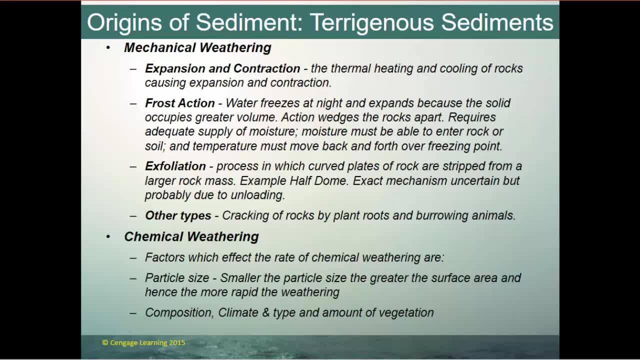 Because it occupies more volume as ice and that wedges the rocks apart and then it melts the next day and then you have a larger opening for more water to run into and freeze and expand that joint again. So basically you have to have a situation where the temperature moves back and forth over. 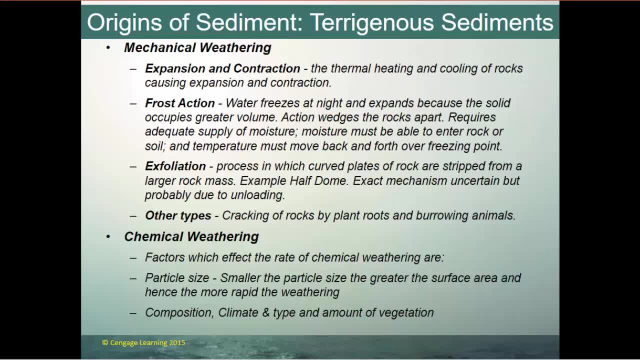 the freezing point and then the freezing and the unfreezing, and freezing and unfreezing of water within a rock will break it into smaller and smaller pieces. Exfoliation is the process in which curved plates of rock are stripped from a larger rock and then they're cut off. So it's a 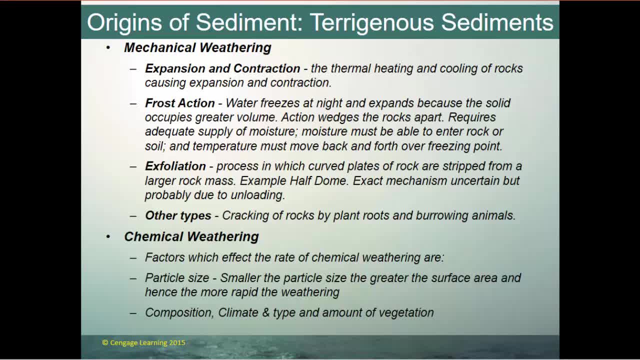 larger mass. An example would be Half Dome. out in California, Yosemite Valley, You have large emplaced plutons of igneous rock. A pluton is because the rock cooled underground and as the material above that rock weathers and it's exposed to the surface, there's less and less pressure on. 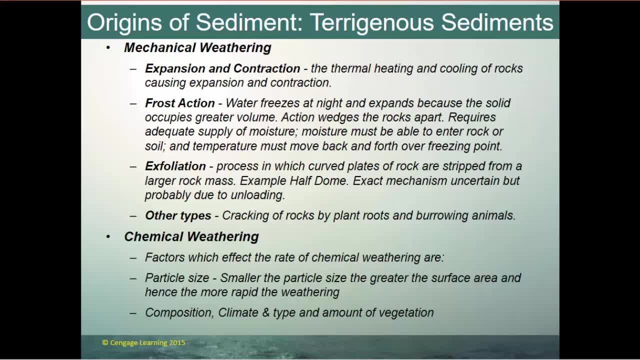 that rock and so it begins to expand upward and it splits, It, shears off, It breaks off in these sheets and those exfoliation sheets break away, and that's the process of chemical weathering. You can also get cracking of rocks by plant roots and burrowing animals. 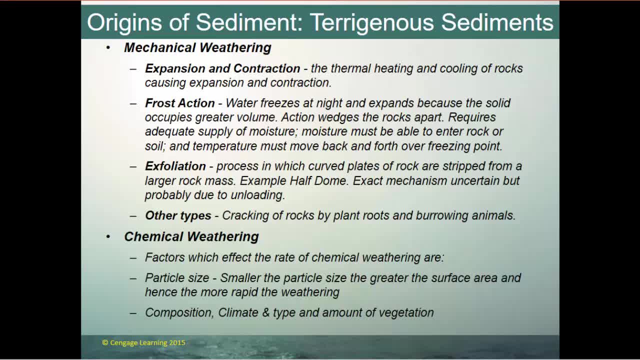 There's chemical weathering, which we talked about. Factors which affect the rate of chemical weathering are the particle size: the smaller the size, the greater the surface and hence more rapid weathering. Composition, climate, different types of vegetation also helped to enhance chemical 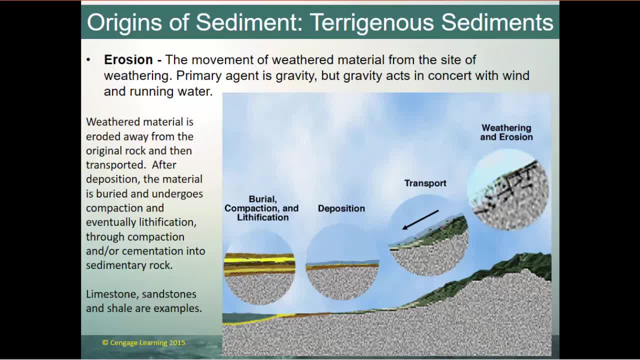 weathering. So once material is weathered then it has to be eroded, and erosion is the movement of weather material from the site of weathering. weathered, it gets broken down into smaller pieces and then something moves those smaller pieces from the site. Typically gravity, wind and water are what cause that to happen. So 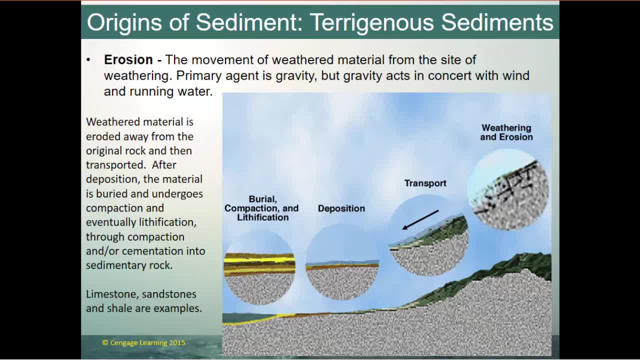 erosion is the transportation of smaller and smaller materials of weathered rock. So weathered material is eroded away from the original rock and then transported. After deposition, the material is buried, and if it's buried deep enough it will undergo compaction where it's squished together. 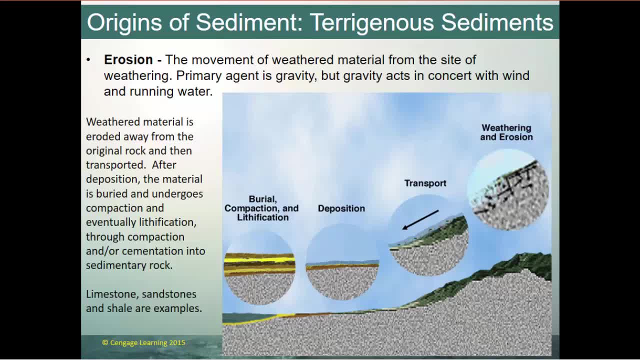 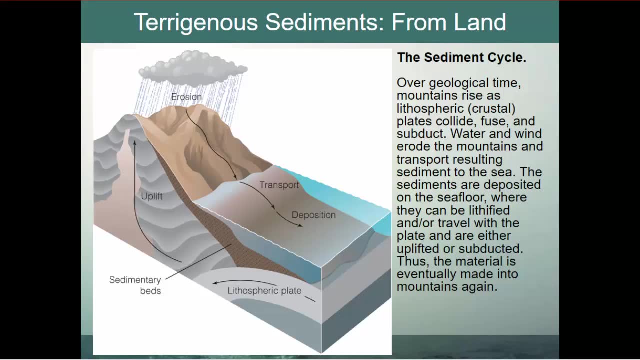 and eventually lithification, which is simply the cementation, the compaction and or cementation into sedimentary rock And limestones and sandstones and shales are all examples of those sedimentary rocks. So this is an example of the sediment cycle You have uplift, of some perhaps. 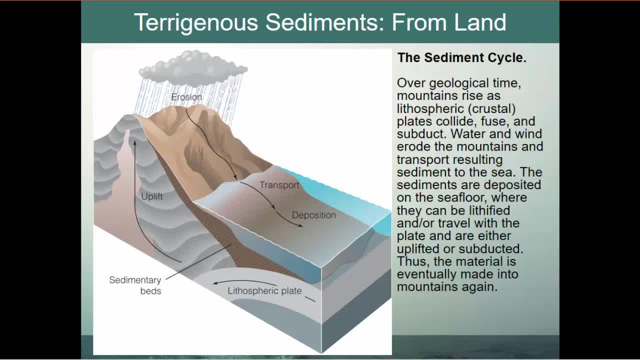 metamorphic or certainly igneous rock, and that uplifted material is exposed to the surface where it is weathered, and then erosion moves it away from the weathered parent. material transportation moves it downslope by gravity, perhaps water is involved and eventually it's. 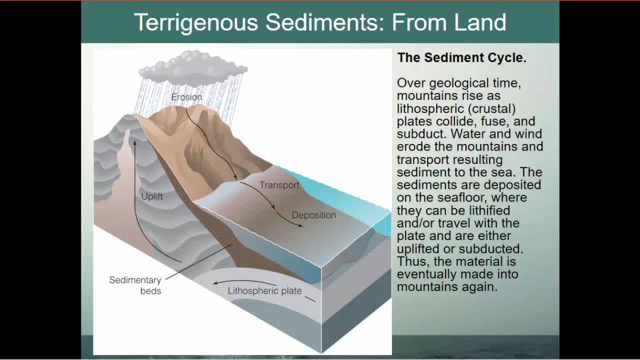 deposited out on the continental margin somewhere, or maybe even out in the abyssal plain and as a layer upon layer is deposited, eventually you may get sedimentary rock that forms and then as lithospheric plates collide, that lithospheric plate where the new sedimentary rock is formed. 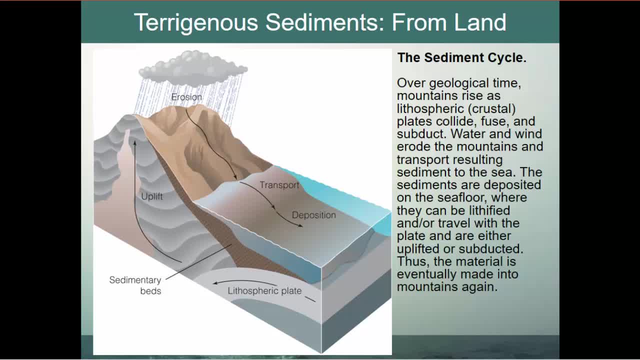 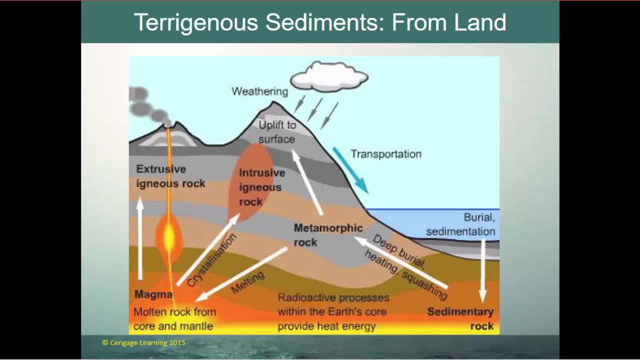 is subducted underneath a continental plate where, once again, you may get some melting and some uplift, And the whole process continues. And this is another, basically example of the same thing, illustration of the same thing: weathering at the top of the mountain, The rock is eroded away. 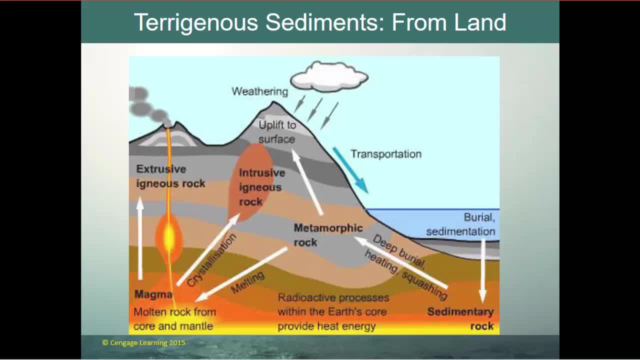 the material is eroded away, it's transported downhill and then out into the ocean, where, eventually, the sediment is buried. Burial and compaction results in sedimentary rock, Now that sedimentary rock may be turned into metamorphic rock or igneous rock or 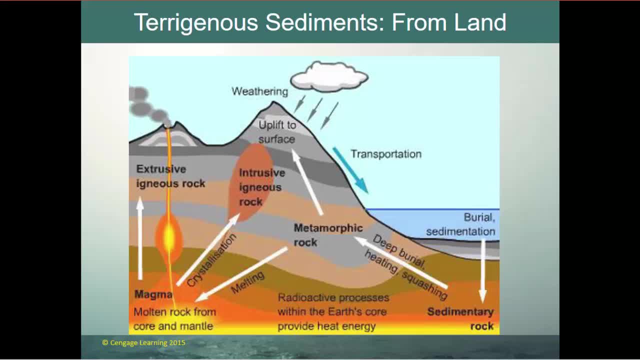 maybe even extrusive igneous rock which cools the surface. but at any rate, in some process, what used to be sediment gets turned into sedimentary rock and eventually gets uplifted as a mountain again, where it once again is eroded Again. that is the the sediment cycle. 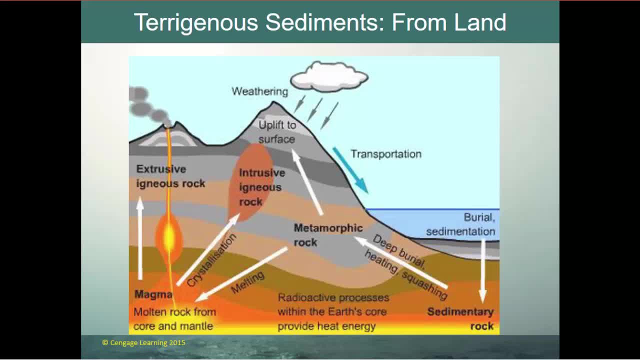 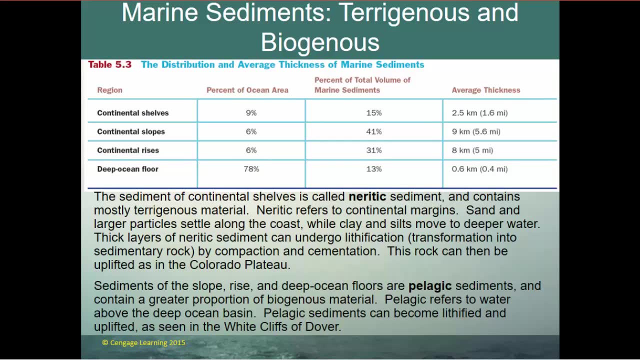 and specifically a terragenous sediment that comes from land. All right, the sediment of the continental shelves is called neuritic sediment and contains mostly terragenous material. Neuritic refers to the continental margins. Sand and larger particles settle along the coast. 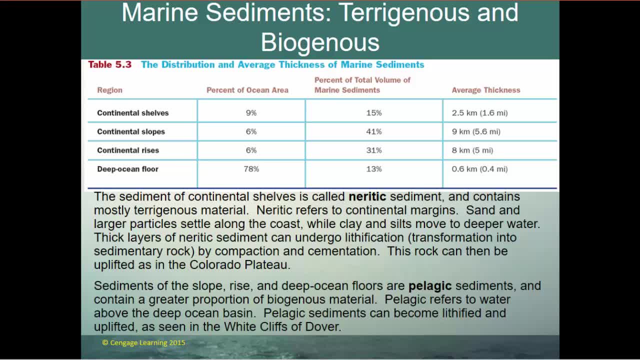 while clays and silts move into deeper water. Remember, as the water slows down, as it moves off the continent, the larger particles are going to fall out first. So first you're going to have sand and larger particles falling out along the coastline: The clays and 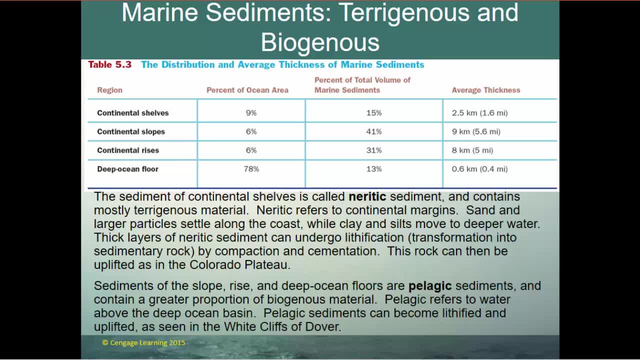 the silts will stay suspended in the water as it moves into deeper and deeper water, and that's where those particles are eventually deposited. So thick layers of neuritic sediment can undergo lithification, transformation into sedimentary rock by compaction, and 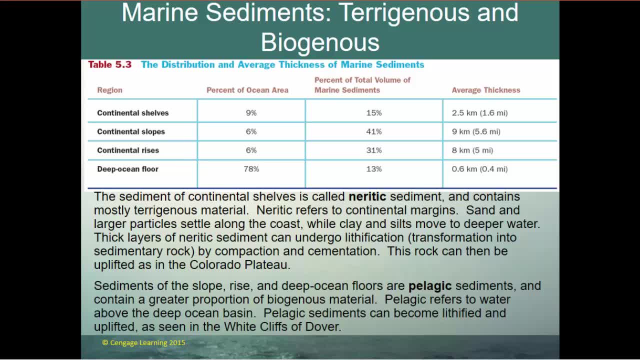 cementation, And this rock can then ultimately be uplifted, And the Colorado Plateau is an excellent example of that. That region of North America, over geologic time, on several occasions was under a shallow sea, where neuritic terragenous sediment was compacted, and 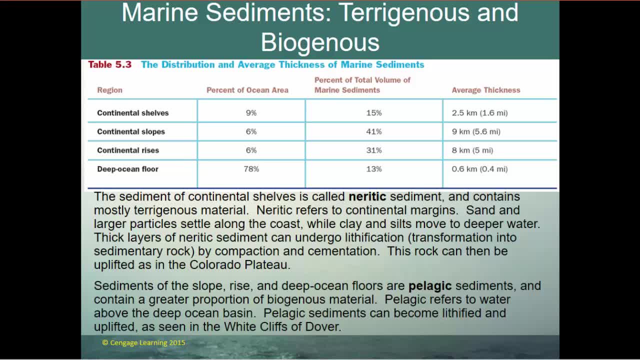 lithified into rock And then at a later date, the entire Colorado Plateau was uplifted and exposed, which is essentially how we got the Grand Canyon. So sediment on the slope rise and deep ocean floor is known as pelagic or pelagic, depending on who's saying it. So it's. 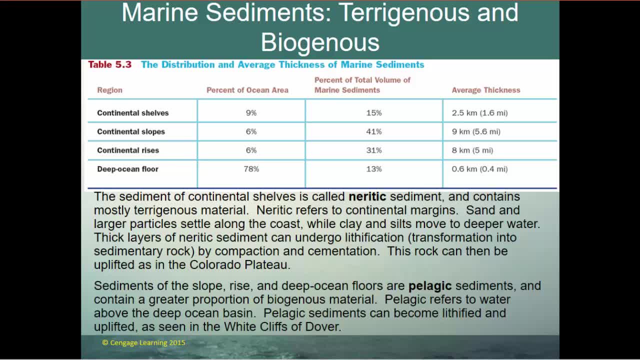 pelagic sediments and contain a greater proportion of biogenesis material. Pelagic refers to the water above the deep ocean basin. So you can remember from Finding Nemo they talked about pelagic sea creatures and neuritic sea creatures. So pelagic sediments can become lithified and uplifted And 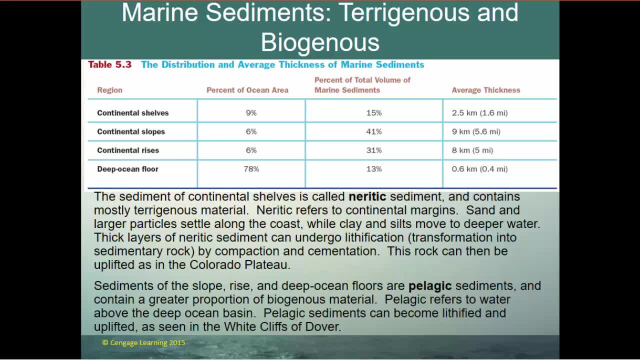 a really good example of that are the White Cliffs of Dover. The White Cliffs of Dover, along the southern edge of the United Kingdom of Britain, England, these massive white cliffs And they are essentially the skeletons of plankton, tiny plankton that accumulated on the seafloor over 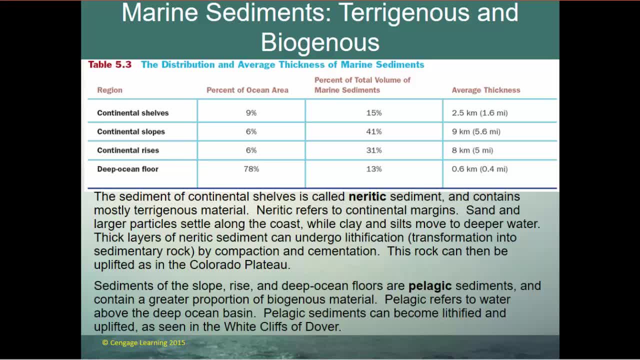 millions of years that were compacted into a sedimentary rock, which is chalk. It's literally a sedimentary rock. All that chalk is just little tiny skeletons of sea creatures, And some type of uplift there pushed that up above the seafloor And that's why it's called the White Cliffs of Dover. 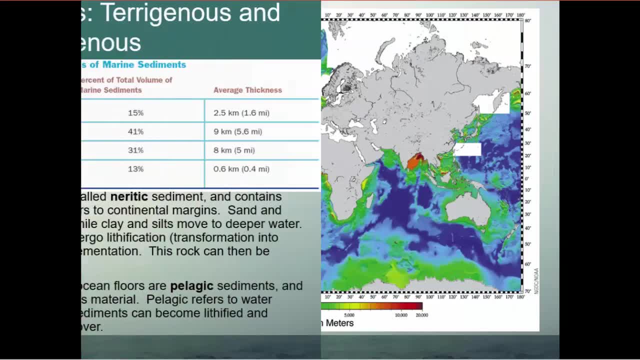 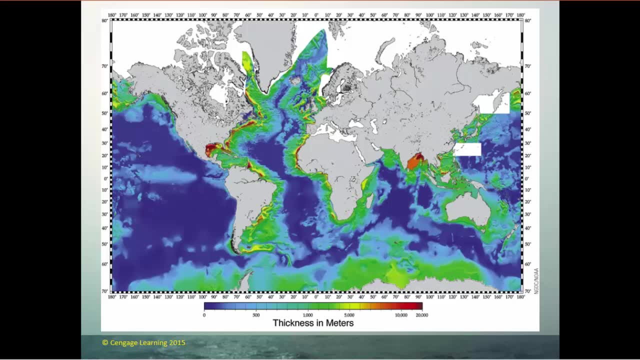 And here we have thickness in meters of the sediments And you can see where the the sediment is thickest is where you get a lot of runoff off the continents, such as in the Indian Ocean, where you get all the runoff off the Tibetan Plateau and comes down the big rivers here. 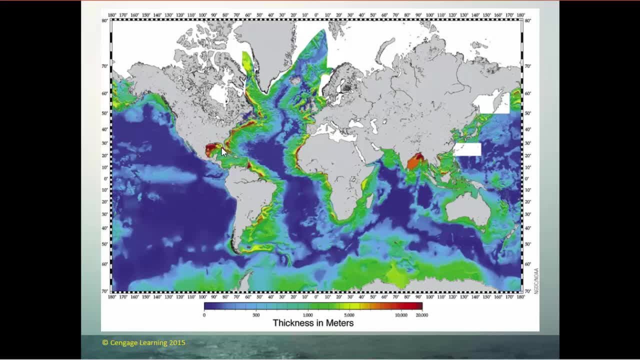 and feeds just a tremendous amount of sediment. We also have a lot of sediment in the Gulf of Mexico because the river is the Rio Grande and mostly really the Mississippi River. that brings sediment, And then the Amazon brings sediment and the Congo brings. 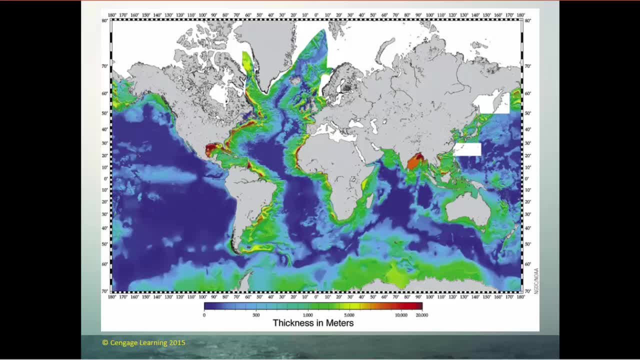 sediment, But where you get a lot of sediment coming off the continent. that's where your, your sediments are thickest on the ocean floor, Then out in the deep ocean, that's where they're thinnest, And again you can see that mid-ocean ridge where new oceanic crust is constantly being. 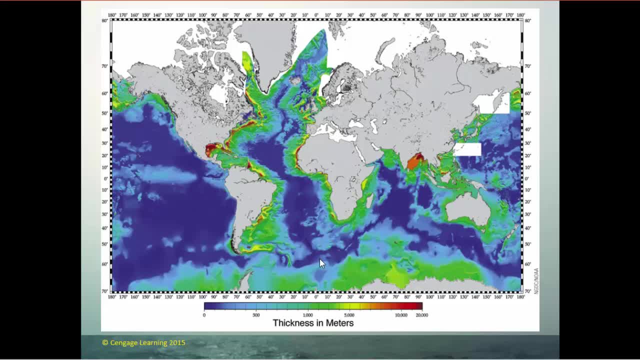 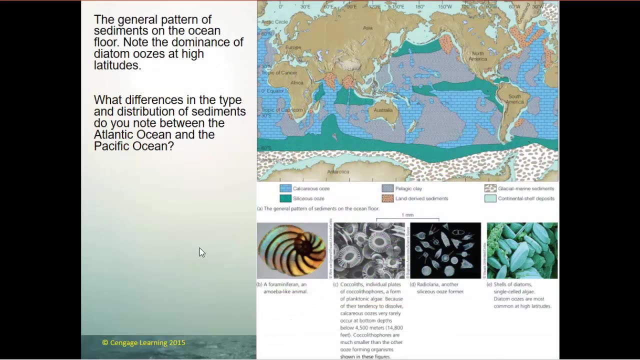 formed. that is where our sediments are the thinnest And this line blue basically follows the Pacific rise and that's where your sediments tend to be the thinnest. So the general pattern of sediment on the ocean floor. you can see the dominance of oozes at high. 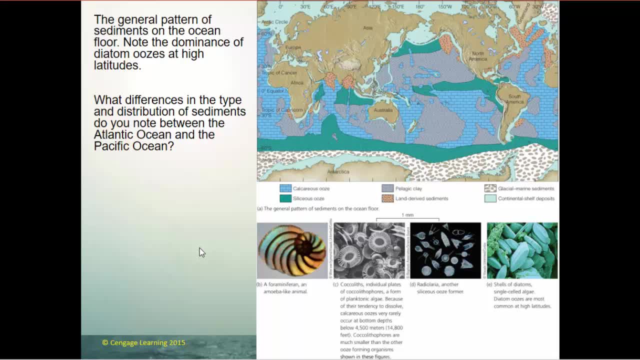 high latitudes And you know, basically, different pelagic environments support different types of biogenous sediment and you get different types of sediments on the seafloor And, of course, those areas that I pointed out as well. these are land-derived sediments. 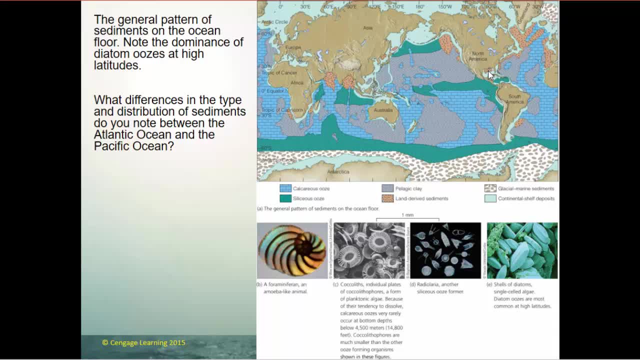 you're going to see that mainly where you have big rivers flowing out into the oceans And you can get a lot of land-derived, and then you get out into the middle of the ocean, you start getting these pelagic sediments, clays and oozes, And then, at higher latitudes, 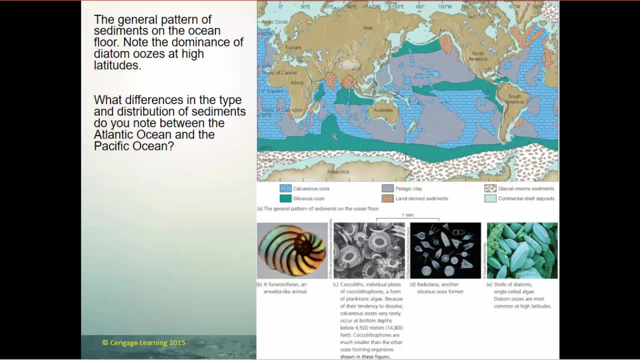 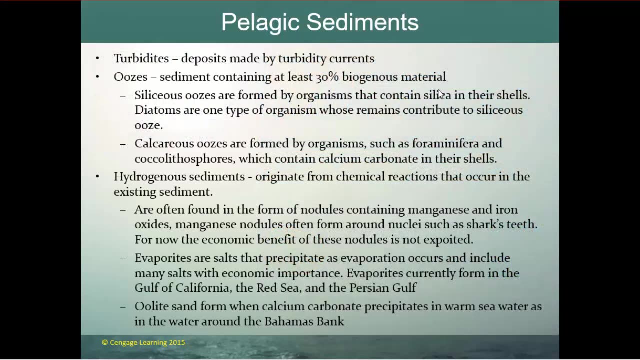 you're going to get these, these silicate derived types of oozes, and it basically is just the marine environment is going to dictate the type of sediment that you can find in different locations and the thickness of that sediment as well. all right, pelagic. 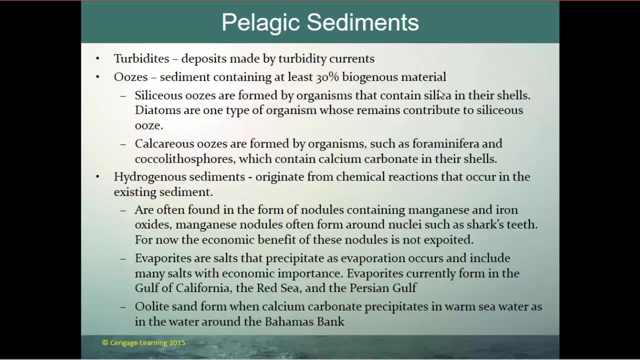 sediments. turbidites are layers of sediment that are created, deposited by turbidity currents. we talked about turbidity currents earlier, where the a lot of sediment gets mixed up, mixed up into the water column, making that area of water more dense, and so it tends to flow downhill where it's deposited at. 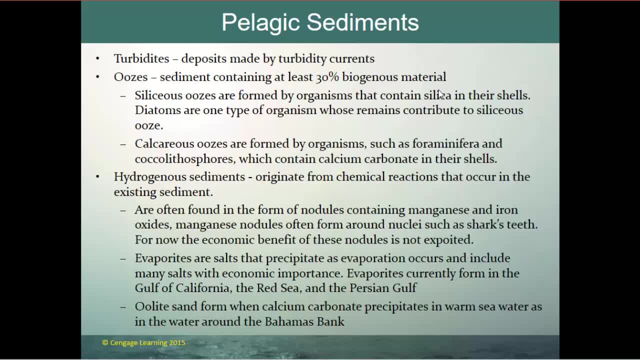 deeper areas. these oozes are sediments that contain at least 30% biogenesis material. so you have the silicate oozes that are formed by organ organisms that contain a lot of silica in their shells. diatoms are one of those organisms who 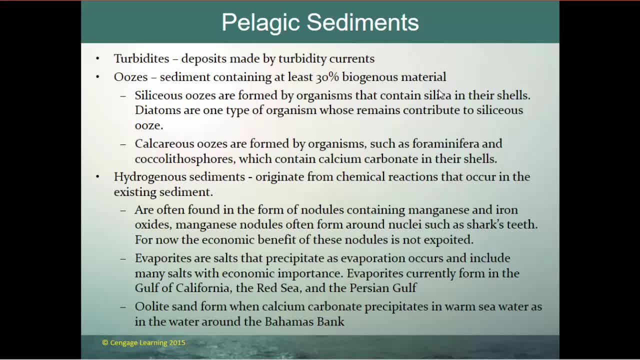 whose remains contribute to silicate oozes. and then calcium oozes are formed by organisms that have a lot of calcium carbonate in their shells. so different types of oozes, based on the different types of sea creatures that die and fall to the bottom of the sea floor and the different types of sea creatures. 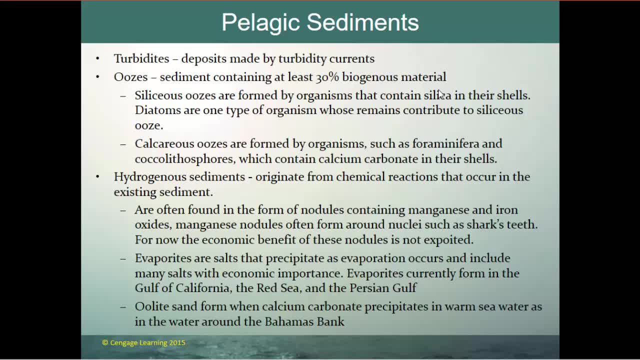 essentially based on the different ocean environment. so hydrogenous sediments. they originate from chemical reactions that occur in existing sediment, so they're often found in the forms of nodules, just little balls containing manganese or iron, and they just they just sort of line around the ocean floor sometimes. manganese nodules often form around nuclei, so something 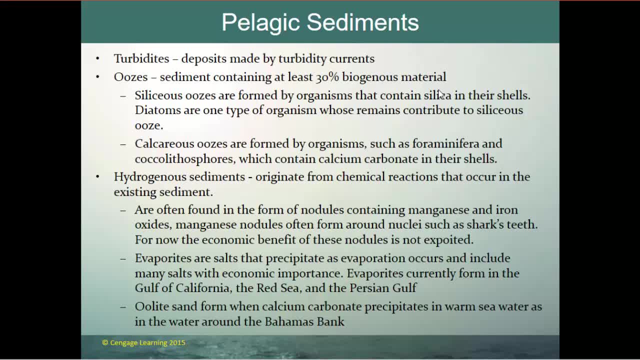 has to be there for the manganese to form around the ocean floor. so that's a little bit of a lahpate, something like a shark's tooth lying on the bottom of the ocean may, because manganese to form around it and you get these little nodules, a vaporites. it's a completely 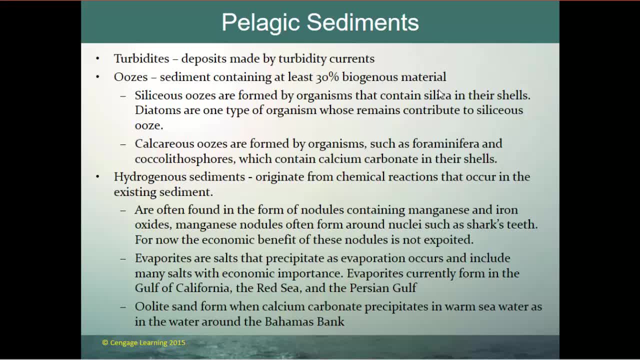 different thing, but it's basically the same process: that the manganese and different in the iron precipitate out of the water. well, evaporites are solids: precipitate out of water as the water evaporates. that's why there are no evaporite shallow ocean, that for some changes in the climate over long periods of time, that shallow ocean or 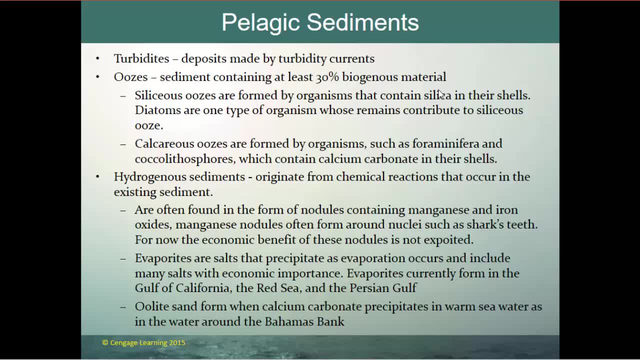 shallow sea begins to evaporate, the salts precipitate out as the water evaporates and they just sort of are left in the bottom of what was the the sea floor. so you can have salts and gypsum and a few other types that usually have some economic importance and 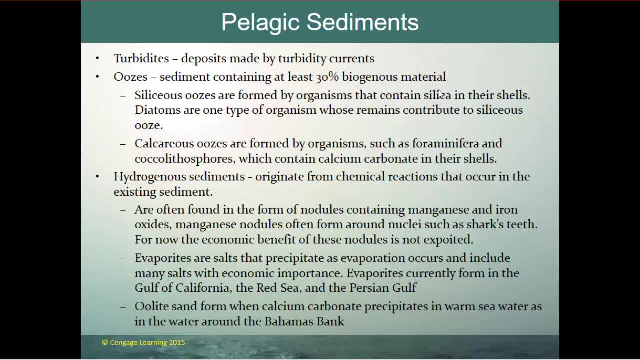 the oolite sands form when calcium carbonate precipitates in warm sea waters and the water like in the water around the Bahama Bank. so the sand is literally not sand like silicon, but it's sand made up of calcium carbonate. we find that the white sands around the Bahama 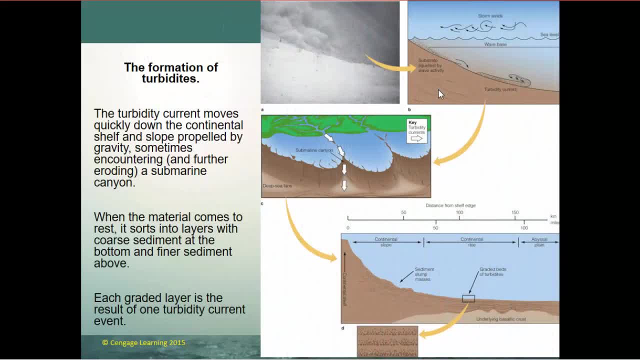 Bank. so we talked about turbidity currents. and again, those turbidity currents move quickly down the continental shelf, propelled by gravity, because the water is more dense, because it contains a lot of um, of different uh sediments in it, and when the material comes to rest it tends to sort. 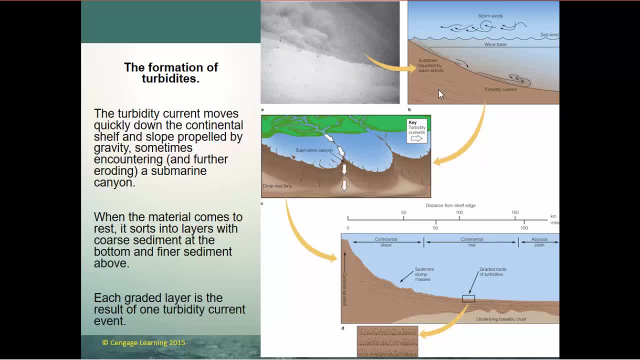 itself into layers, with the coarser sediment falling out first. so the coarser sediment is going to be at the bottom and the fire sentiments on top, and each graded layer is the result of of one turbidity current. so we'll get these different layers with uh course to find and 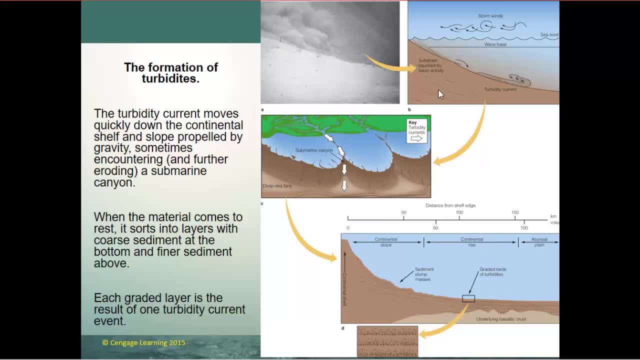 course, to find the course of findings in the very bottom illustration. and, uh, you know, one turbidity current sends down one layer. the second turbidity current much later sends down the second layer, and that gives us an idea of what had happened in that, in that region. all right, so. 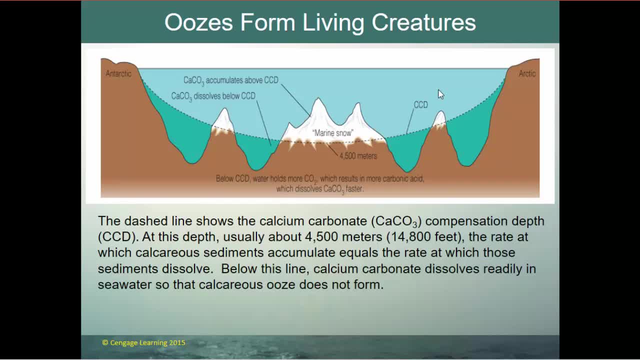 here the oozes, sometimes called marine snow. the dashed line shows the calcium calcium carbonate compensation depth, the ccd. at this depth, usually about 4 500 meters, the rate at which calcium sediments accumulates equals the rate at which the calcium carbonate dissolves. so 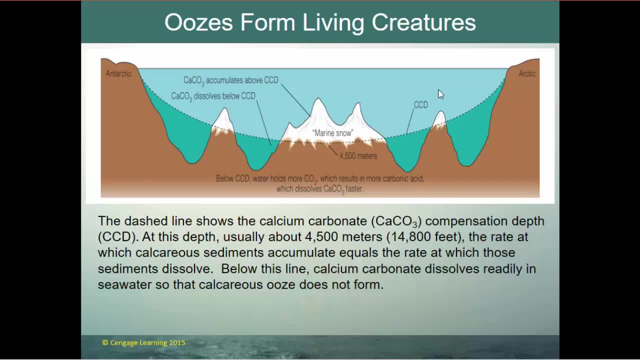 things dissolve will dissolve more readily in the colder water. so below this line the calcium carbonate dissolves readily in the seawater, so you don't get any oozes that form. above that line the calcium carbonate doesn't dissolve in the seawater as well, so you get an accumulation. you. 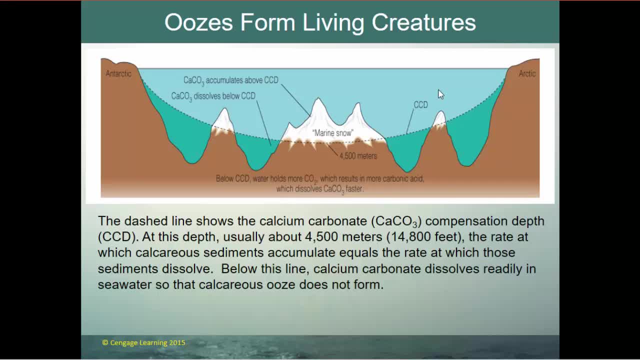 get those marine, marine snows. and, um, you know, below the ccd water holds more, more co2 because gases dissolve more easily in colder water and that results in more carbonic acid which dissolves more the calcium carbonate faster. so above that 4500 meter line there's less co2 in the water, which 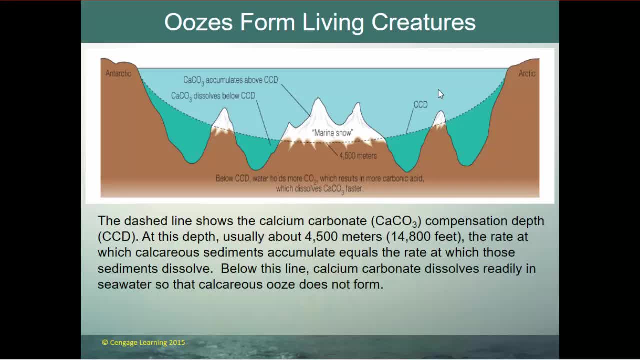 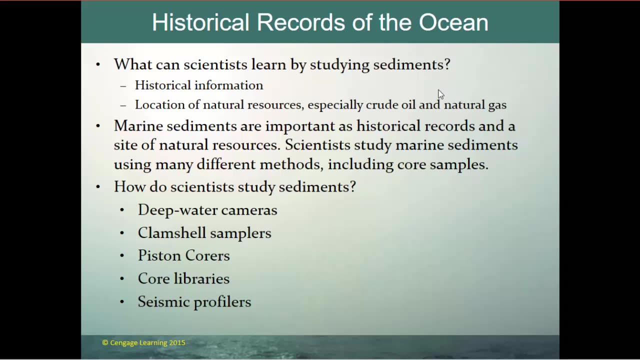 means there's less carbonic acid in the water, which means the um, the calcium carbonate, the calcium shells. they don't dissolve and they they rain down on the sea floor as a marine snow. so what can we learn by studying sediment? historical information, the location of natural resources like oil and natural gas. marine sediments are important as historical records. 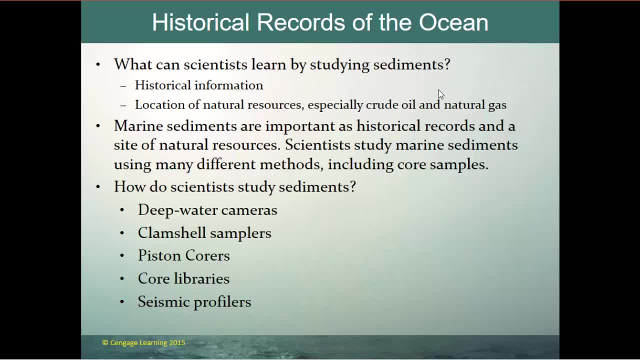 and the site of natural resources. scientists can study marine sediments using many different methods, including just simply taking core samples, where they just dig down deep and and get a core sample and taking a look at that core sample with depth will give us an idea of what has happened. 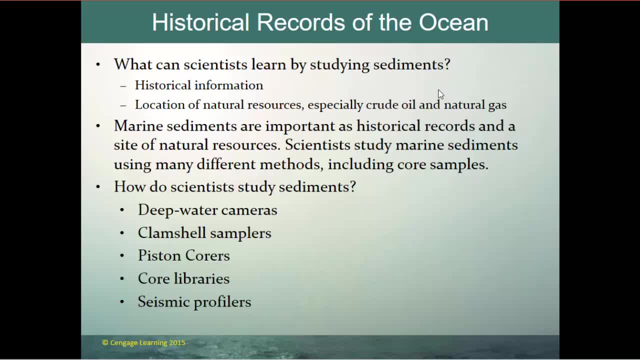 historically back in time in that marine environment. so some of the ways, of course, scientists get their observations- they have cameras and clamshell samplers and cores and seismic profiles and things like that. so that's one of the things that we're going to be looking at today. 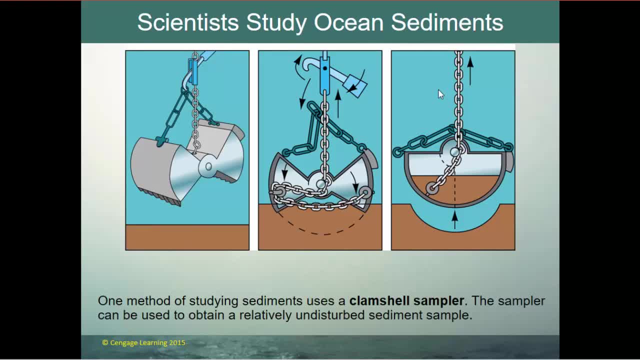 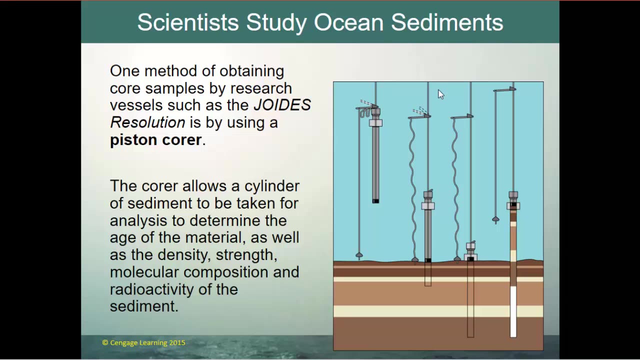 just lots of ways they can get information out of the sediment. so this is one method. that's: the clamshell sampler just reaches in, scoops up a big, uh big scoop of sediment to take back and study. and then here is a method by which they get a cores and again you can see that it lands in the 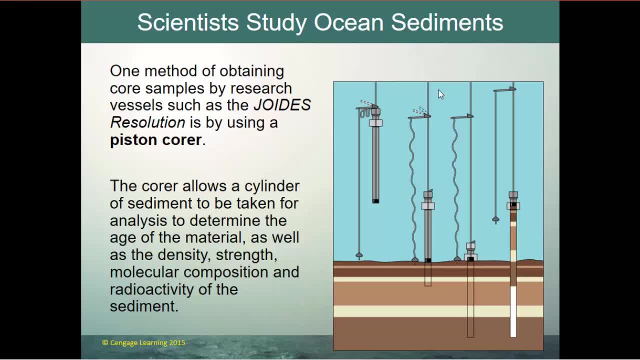 sea floor and it digs down and each subsequent layer, subsequent layer of sediment as you get deeper and deeper beneath the sea floor came from a period longer and longer ago, and so this is one method that we're able to sample what's happening on the sea floor um and know what happened. 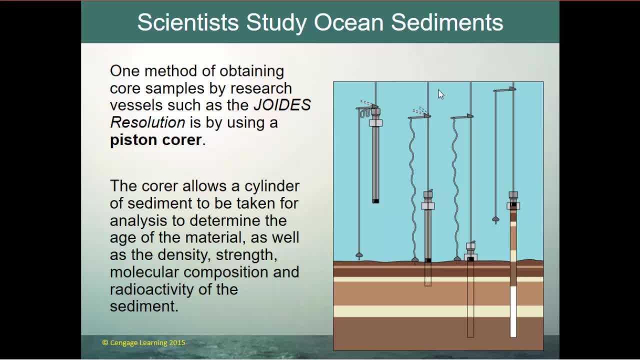 historically so. this is one method of obtaining core samples. it's called the piston core. the core allows the cylinder of sediment to be taken for analysis to determine the age of the material, as well as the density, strength, the molecular composition of the radioactivity in the sediment. 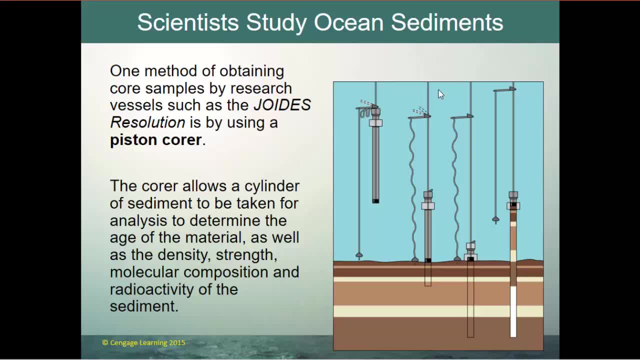 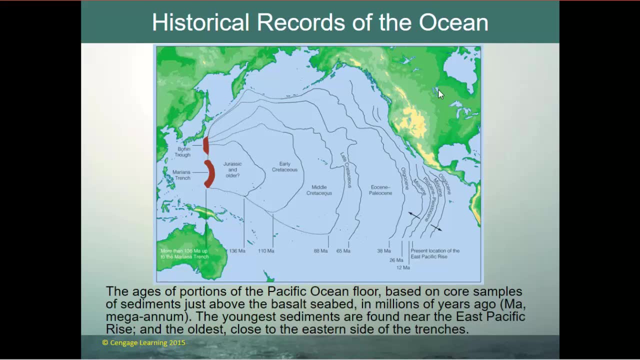 so you pull the sediment up, you radioactively age it and then you know what was happening in the marine environment above that area, um based on- and it is, and it's a very, very good way to get a climate history, whether it was cold or warm in the past. all right, we talked about um, the mid-ocean ridge in the pacific ocean being 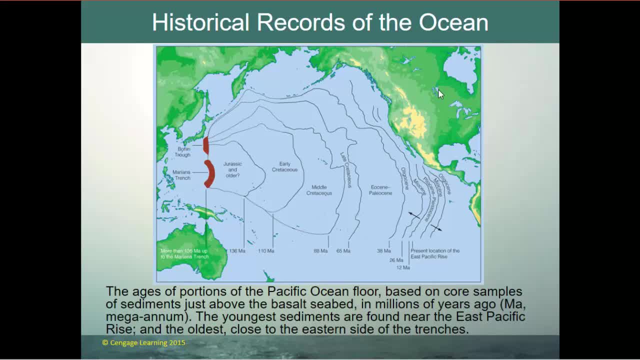 displaced well to the east and so the youngest rocks on in the pacific are in that, along that mid-ocean ridge which basically comes from the baja of california south into the southern pacific ocean, and that's where the youngest rocks are, where it says present location of the east pacific. 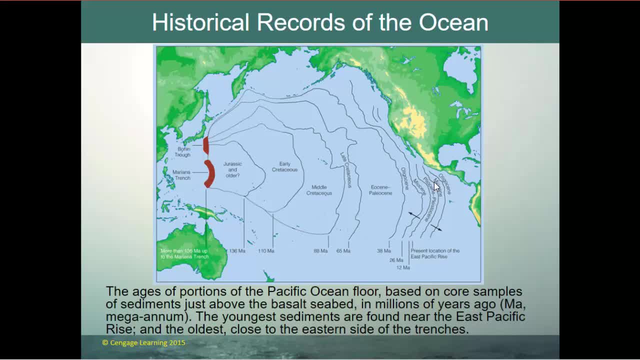 rise right here. so this is the east pacific rise right in here, and everything as you go away gets older: a stripe of of rocks in the miocene between 12 million 26 million years ago, on the west of it and on the east of it, and then a stripe of rock from the um oligocene, which would be 26 to 36. 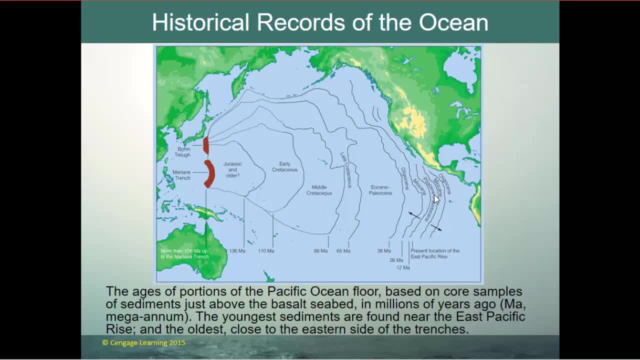 million years and that, and these stripes are moving away as new seafloor is formed and you get older and older. so lake cretaceous. so this is about the time, uh, when the dinosaurs were, uh, caused to become extinct, very likely from a comet or an asteroid that struck the earth- probably a comet, but could have been a really. 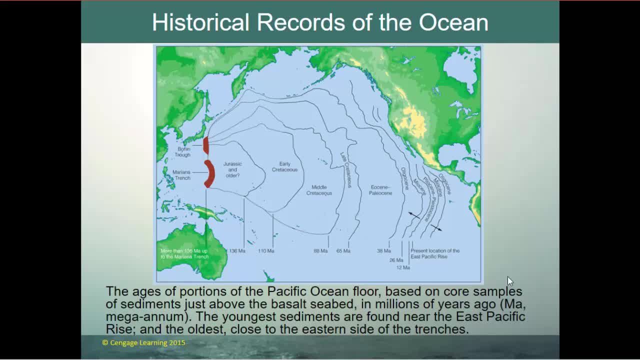 big asteroid. um, so what that means is that 65 million years ago, this, this stripe of rock, was being formed along the east pacific rise and then moving away, and it gets older and older and older, and, and where we start to see a change in the age is where 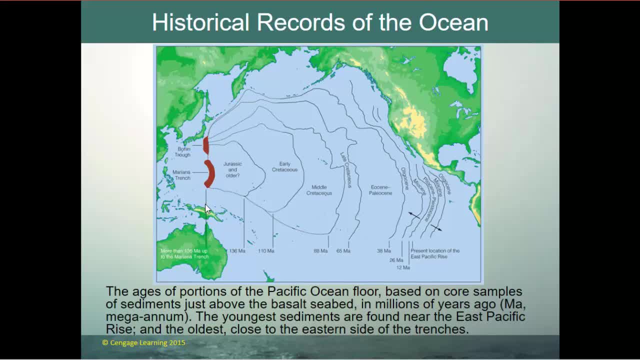 the pacific plate begins to change and it starts to change, and it starts to change, and it starts to change and it begins to subduct under other plates, and this is one of those subduction zones where we get these deep trenches, and this is another subduction zone, and at this subduction zone, the 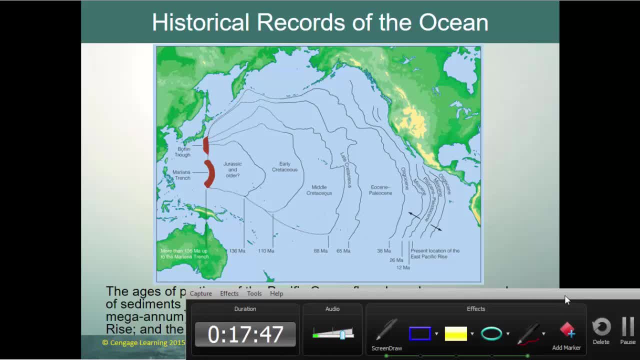 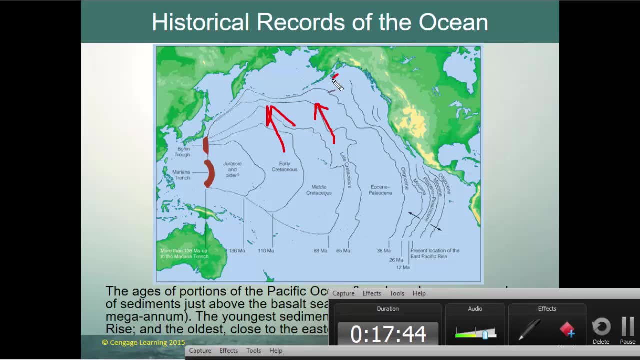 pacific plate is: uh is moving underneath this uh the plate to the north, and so the the pacific plate is moving like this and it- this is the subduction zone here, and so on the back side of the subduction and the plate goes under again. that's the old, uh, the the younger plate. this is the older. 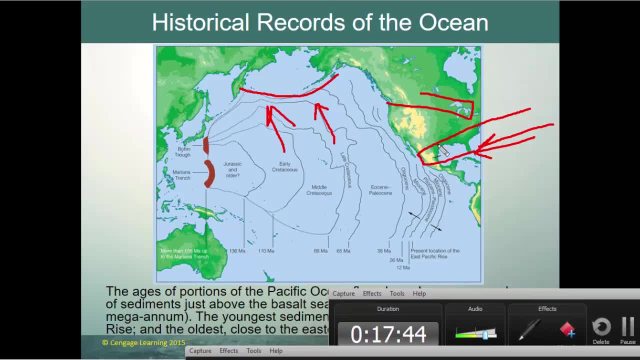 plate going down, and so this is the direction we're talking about and the melting of this. this magma wedge is where you get volcanoes that form. so, as this plate subducts down, volcanoes form the aleutian island chain here, the same way they formed these island chains here as this subduction was. 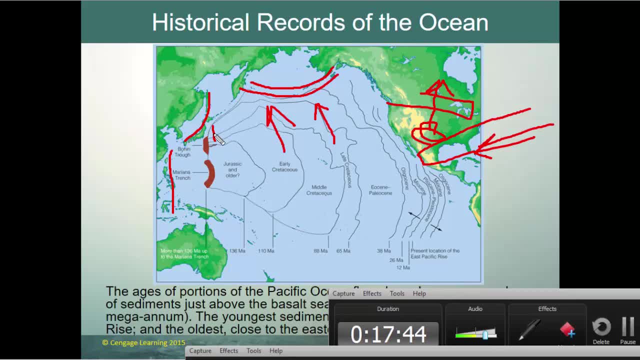 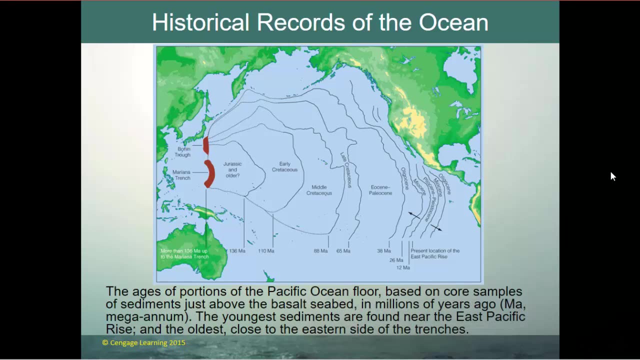 occurring, but the current day subduction is happening here and these trenches here are. are this, this feature that gets formed when plates subduct, one subducts under the other, and so again, the explanation for all these geologic, geologic features basically always comes from plate. 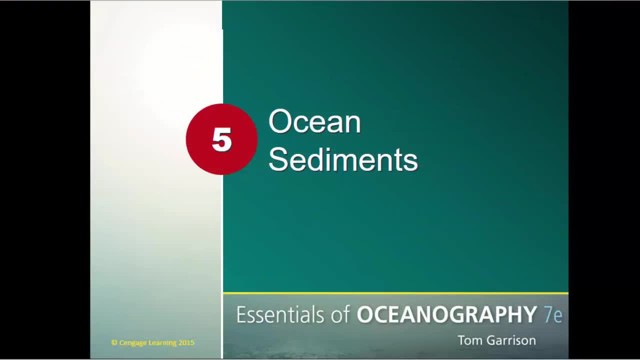 tectonics. so that wraps up chapter five on ocean sediments. we'll be moving on to chapter six next time, and chapter six is on water and ocean structure. so we'll be talking about the, the physical structure of water, of h2o and the fact that it's a very powerful solvent, and how the